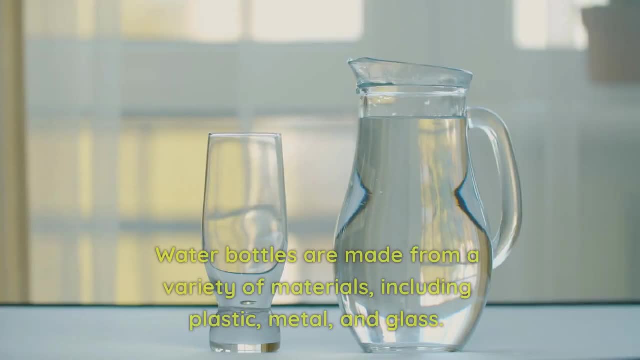 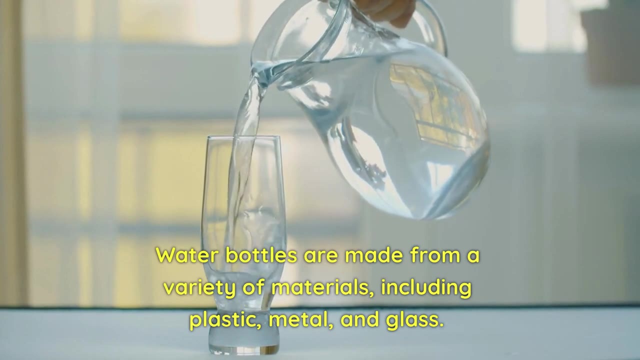 The water bottle is designed to keep your water nice and cold. The water bottle is designed to keep your water nice and cold. Water bottles are made from a variety of materials, including plastic, metal and glass. Each material has its own unique properties which make it better suited for certain applications. 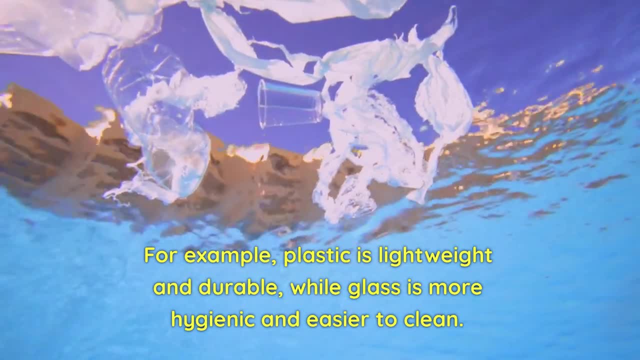 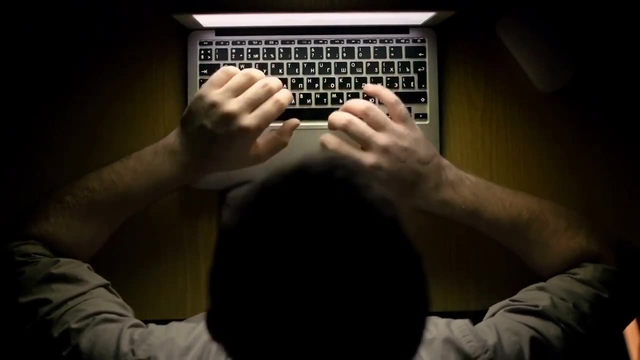 For example, plastic is lightweight and durable, while glass is more hygienic and easier to clean. For example, plastic is lightweight and durable, while glass is more hygienic and easier to clean. Next up, let's talk about keyboards. 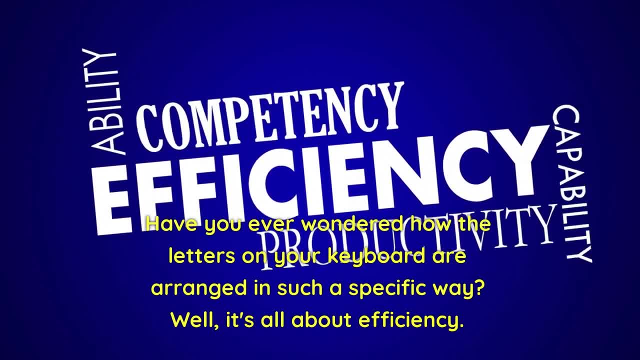 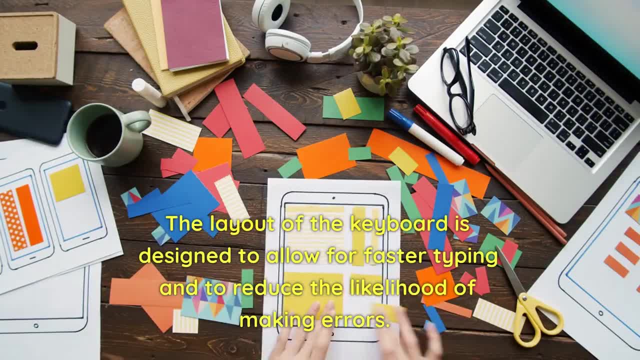 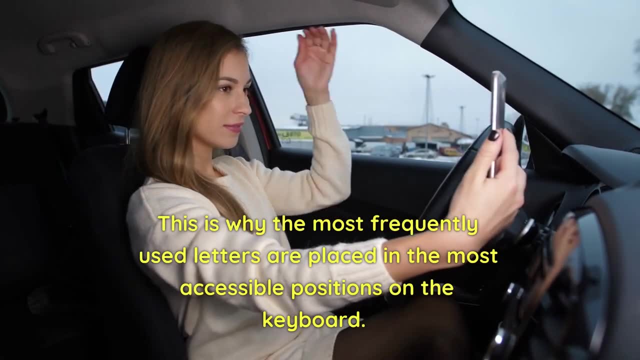 Have you ever wondered how the letters on your keyboard are arranged in such a specific way? Well, it's all about efficiency. The layout of the keyboard is designed to allow for faster typing and to reduce the likelihood of making errors. This is why the most frequently used letters are placed in the most accessible positions on the keyboard. 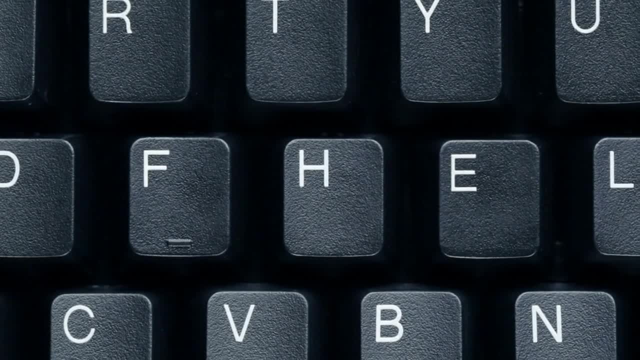 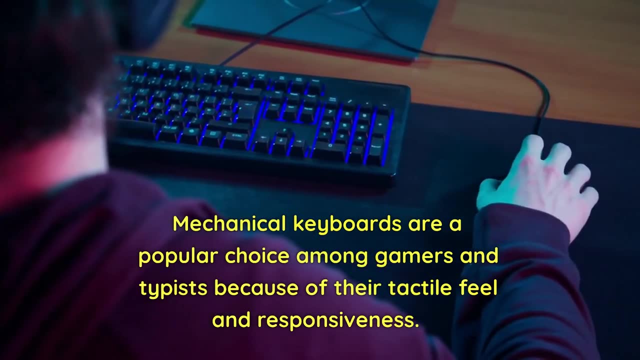 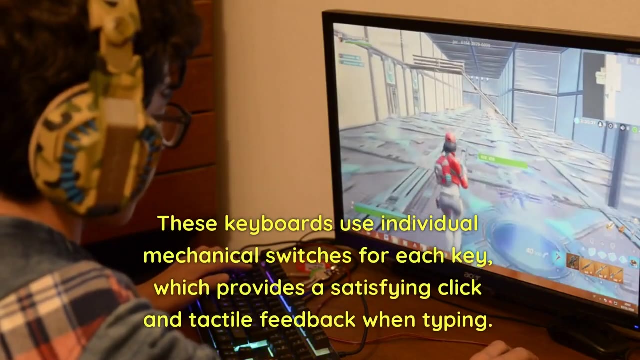 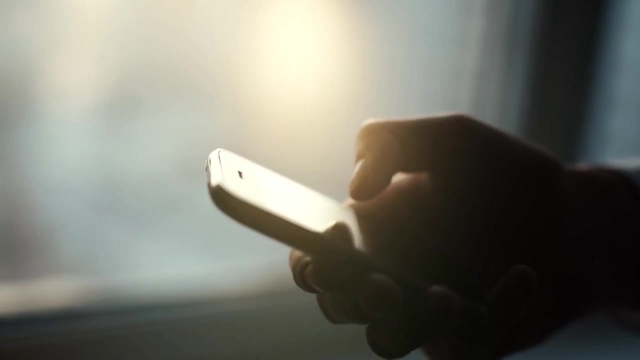 This is why the most frequently used letters are placed in the most accessible positions on the keyboard. Mechanical keyboards are a popular choice among gamers and typists because of their tactile feel and responsiveness. These keyboards use individual mechanical switches for each key, which provides a satisfying click and tactile feedback when typing. 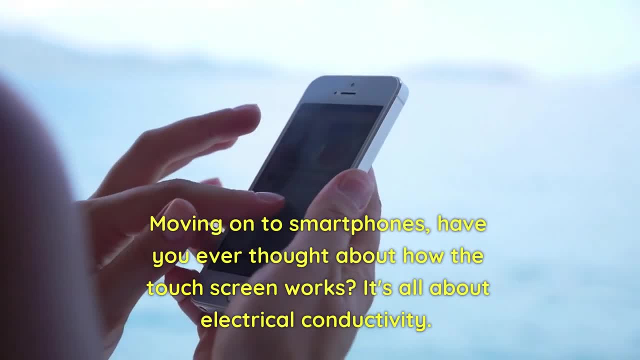 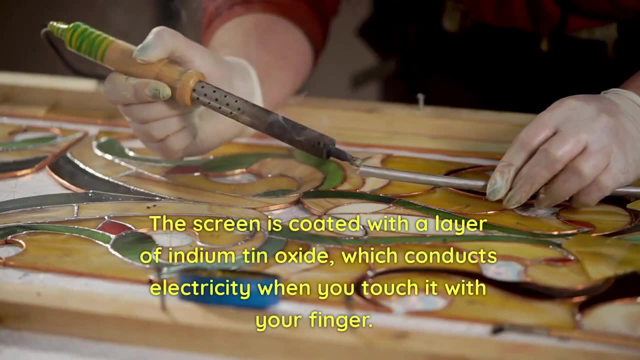 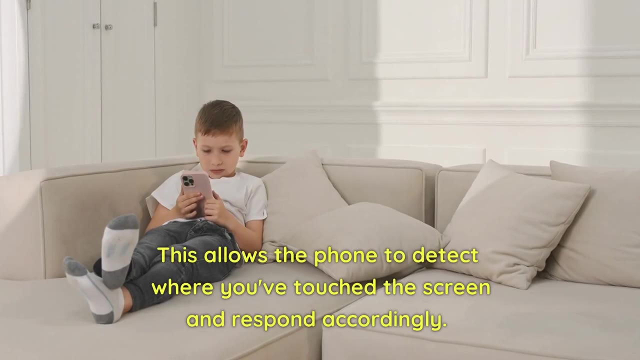 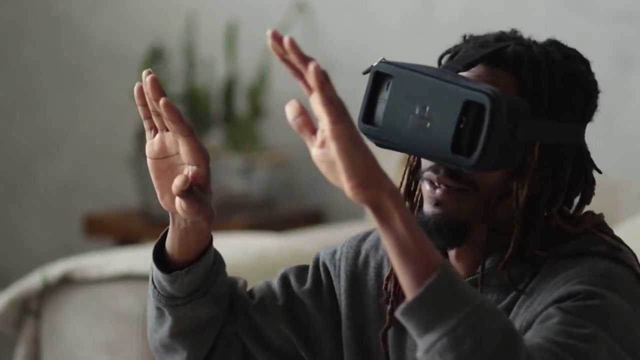 Moving on to smartphones, have you ever thought about how the touch screen works? It's all about electrical conductivity. The screen is coated with a layer of indium tin oxide, which conducts electricity when you touch it with your finger. This allows the phone to detect where you've touched the screen and respond accordingly. 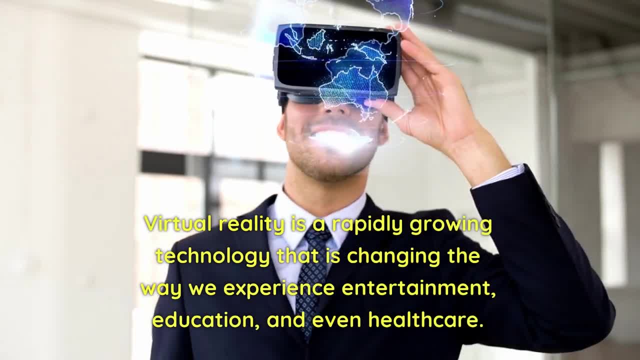 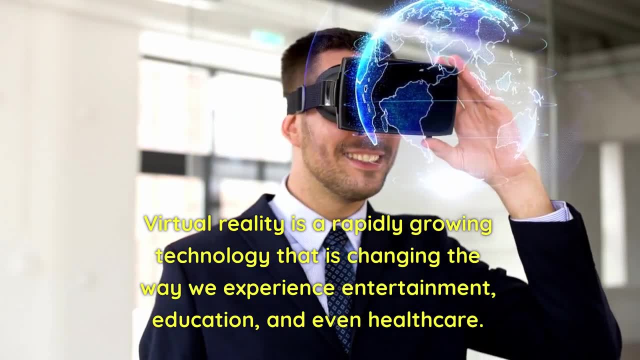 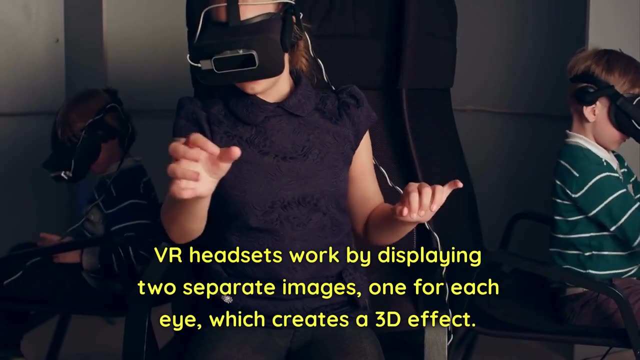 Virtual reality is a rapidly growing technology that is changing the way we experience entertainment, education and even healthcare. VR headsets work by displaying two separate images, one for each eye, which creates a 3D effect. These images are displayed on screens positioned close to the user's eyes.